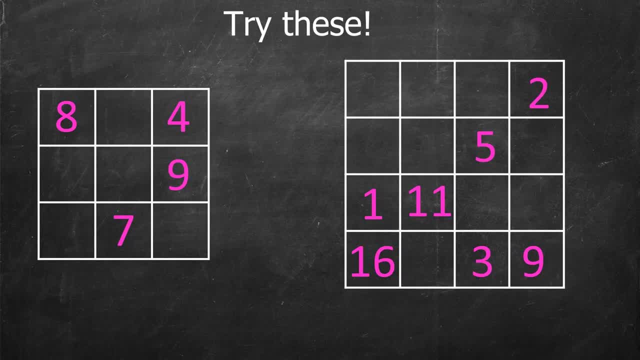 And the way these are commonly presented is actually a puzzle. If I give you either a 3x3 or a 4x4 with a bunch of the numbers missing, you have to figure out how can you fill that in to create the magic square. 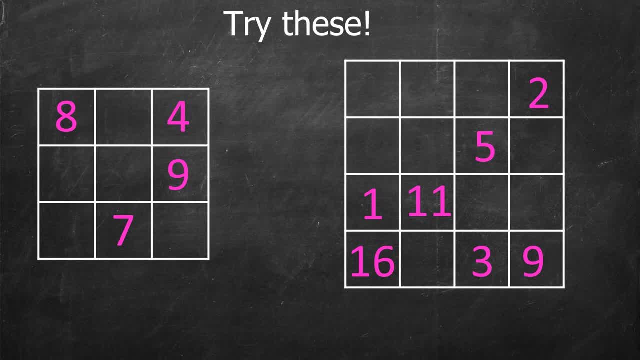 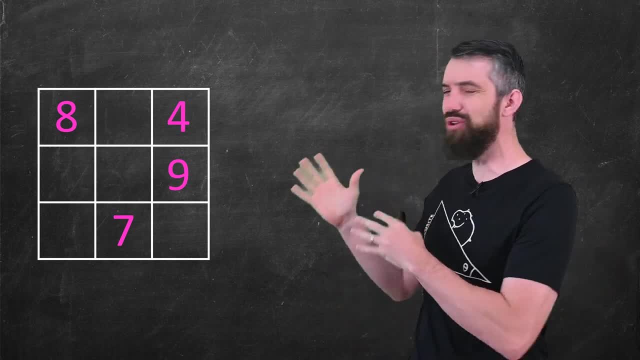 I'd encourage you to pause the video. Try it out yourself. Can you figure out what the missing numbers should be? Even though these are magic squares, mathematicians do reveal their secrets. so let's try to figure out the 3x3 one. 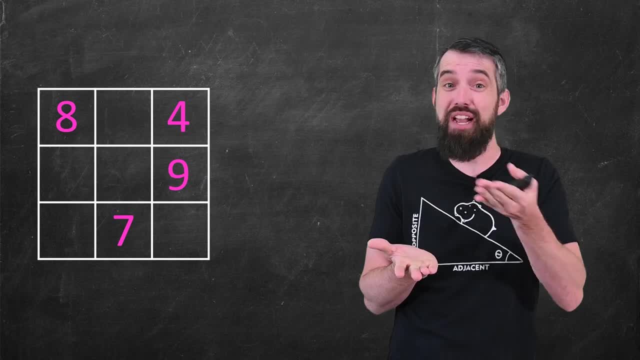 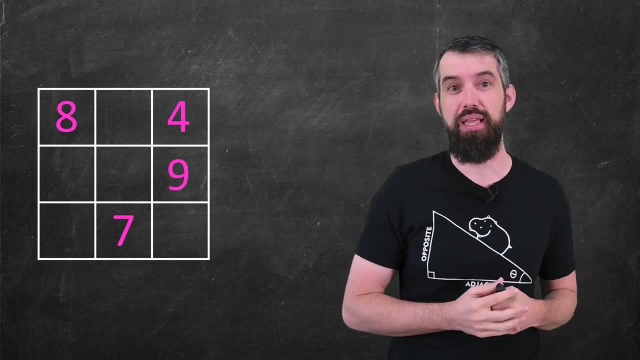 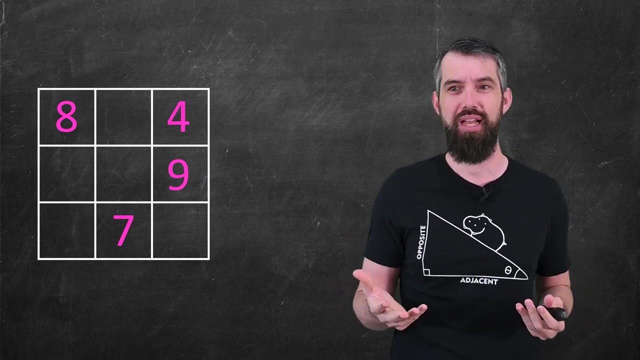 Because there's six unknowns. I don't want to do all six factorial guesses, I don't want to brute force this. Well, by the end of the video we're going to have really powerful tools to do this. basically, immediately, I want to show how you might do it in sort of an ad hoc way, knowing nothing beyond just the basic rules. 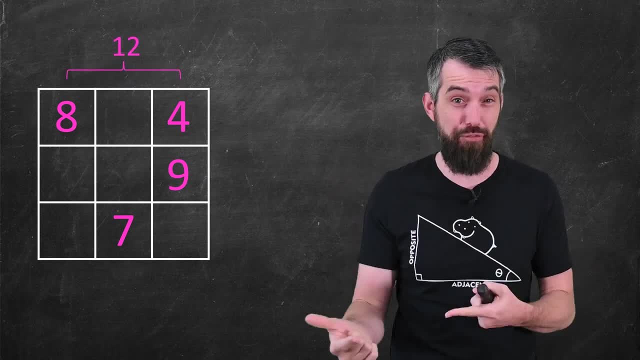 For example, when I was doing this, I was trying to figure out what the missing numbers should be. For example, when I was doing this, I noticed that the top row had an 8 and 4, which added up to 12,, and that the right column had a 4 and a 9 that added up to 13.. 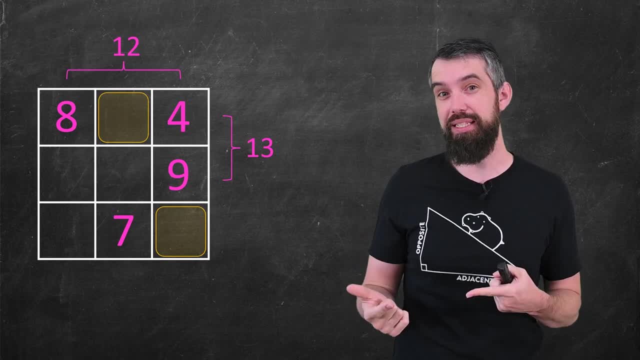 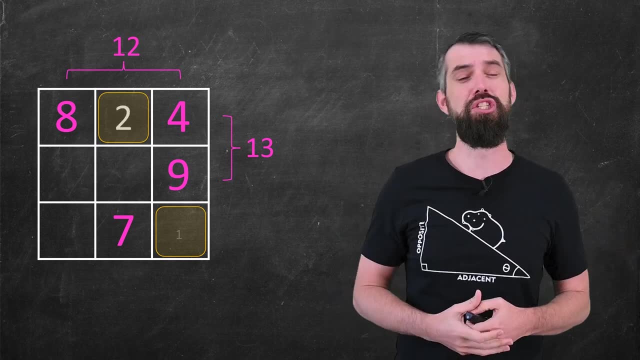 And so, when it came to filling in the two remaining pieces, I knew that the one in the top row had to be one bigger than the one in the right column, So like something like 2 and 1 would work, or 3 and 2.. 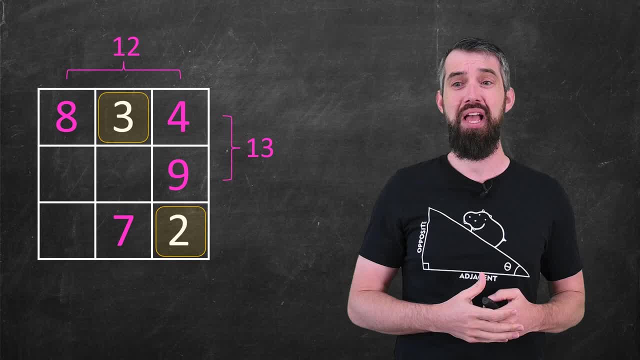 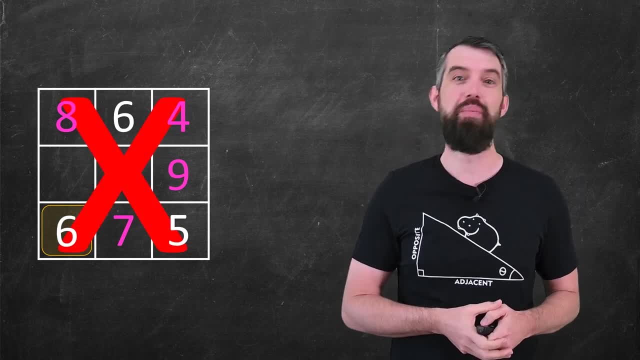 That means that there's a 6.. We've already used 6.. This doesn't work, But it turns out. one of the other ones does 3,, 2,. if I now do, the bottom row gets a 6, and that's totally fine. I can do that. 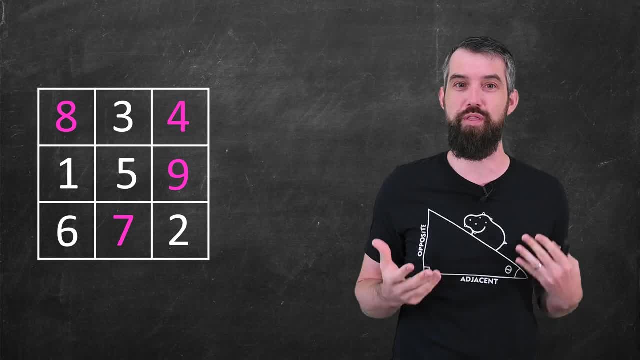 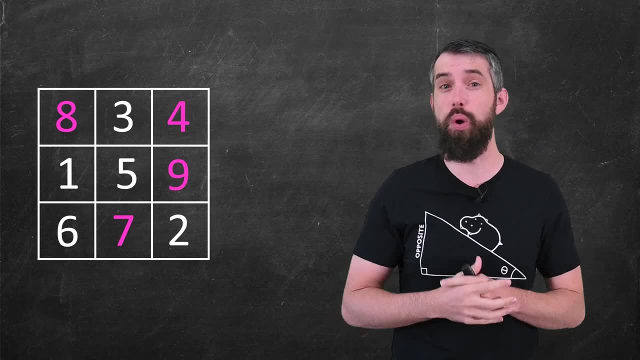 And then you just fill in the remaining spots. That forces the 5 in the middle. It forces the 1 in the remaining spot. You can check it. This is a magic square, But there's no guarantee that ad hoc method is going to generalize to all of these puzzles. 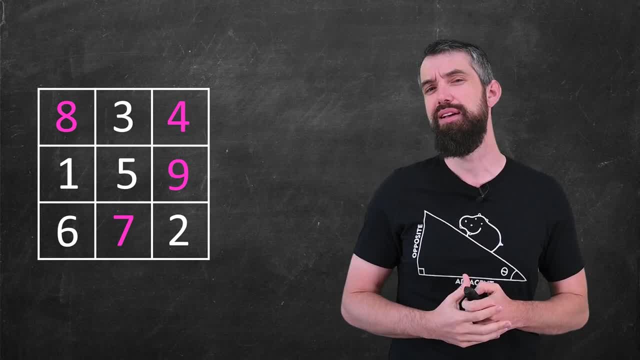 and certainly gets more complicated in the 4x4 case, if you tried that one. So what can we do? Well, in this video, what I'm really going to lead to. Well, in this video, what I'm really going to lead to. 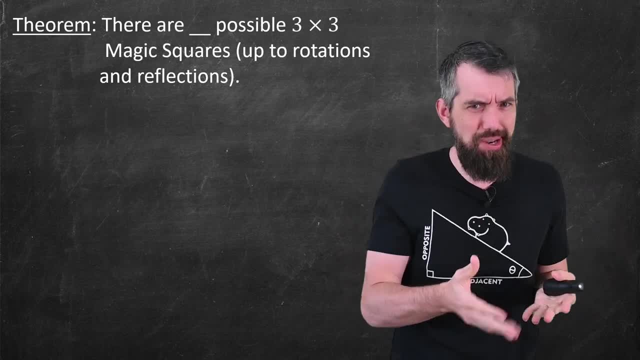 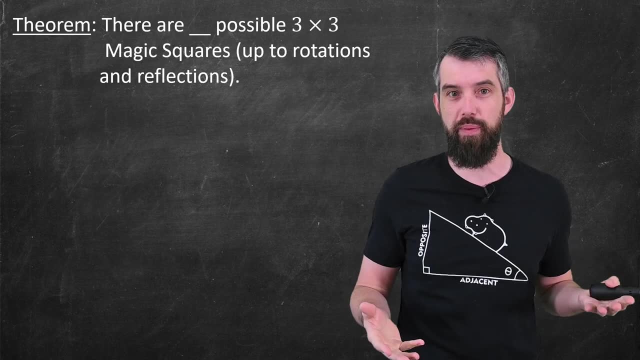 is a theorem that says there are some number- we'll figure out the number as we go along- of possible 3x3 squares, up to rotations and reflections. We'll talk about those Now. if you want to pause and try to prove this theorem all on your own, I encourage you to do that. 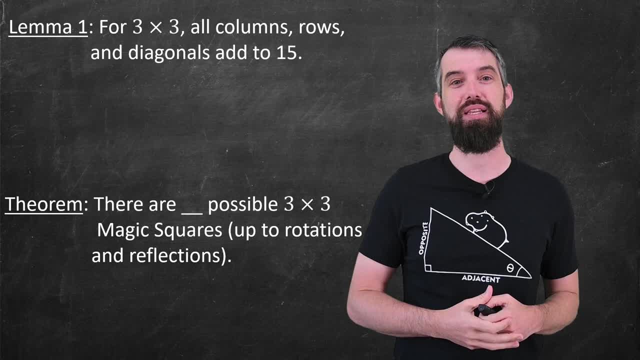 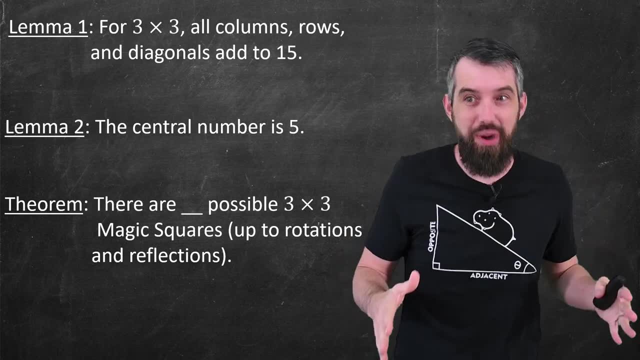 But for spoilers, I'm going to break it up with a couple different lemmas. I'm going to first show that the addition of the rows to 15, like we saw in the examples- always happens. It's always going to add up to 15.. 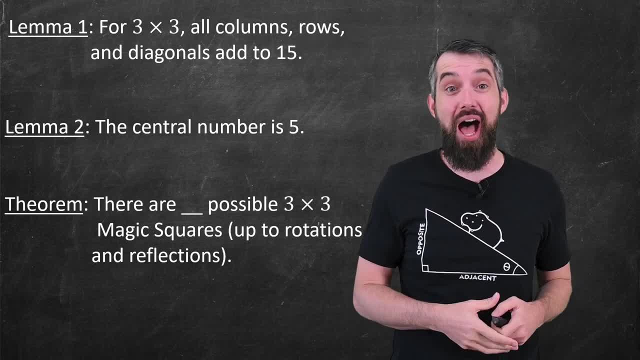 And secondly, you might have noticed in our example. And secondly, you might have noticed in our example the center thing was always a 5.. And again, that is also a lemma. The center number always has to be a 5.. 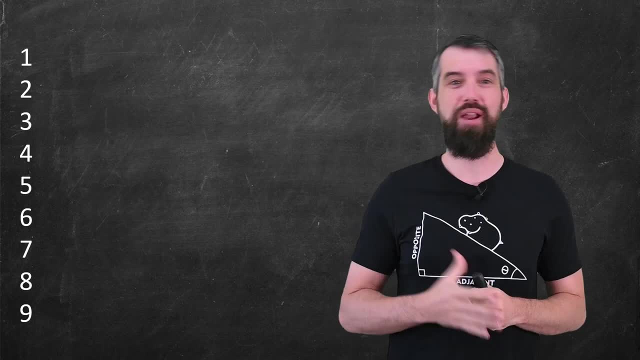 To prove our lemma, we're going to need to know the sum of the numbers between 1 and 9, which you could compute out if you so wished, But I want to show you, as a side tangent, a really fast way to be able to do this. 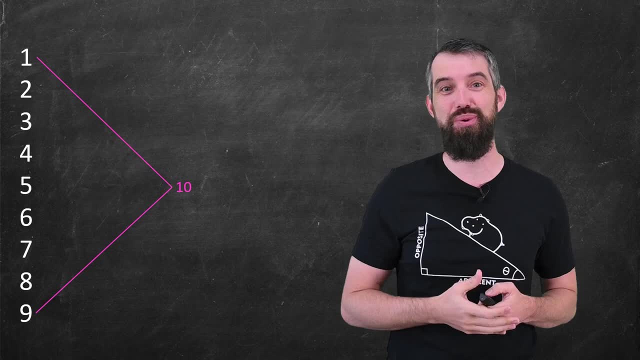 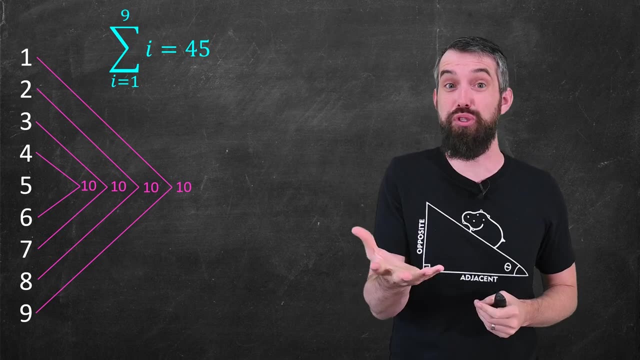 I noticed that the 1 and the 9 add up to 10, as does the 2 and the 8,, as does the 3 and the 7, and the 4 and the 6. And, as a result, the sum of the first 9 numbers is just the 4 tens, which is 40,. 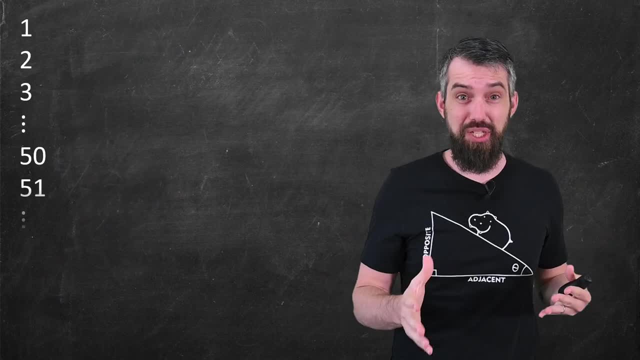 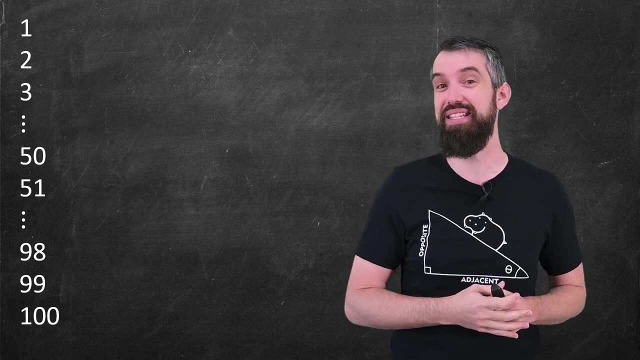 and the 5, which was left out, 45.. There's an infamous story about the great polymath Gauss, who was able to, in elementary school, add up 1 to 100, using basically this exact same trick incredibly quickly. 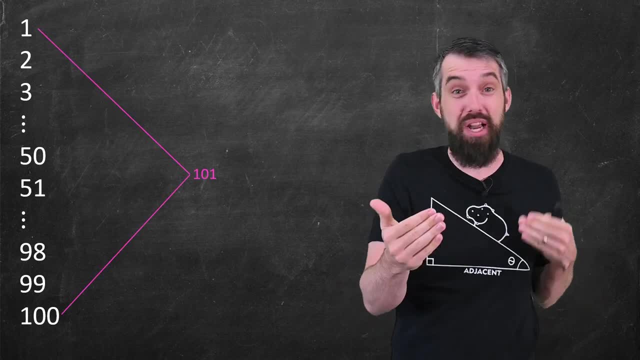 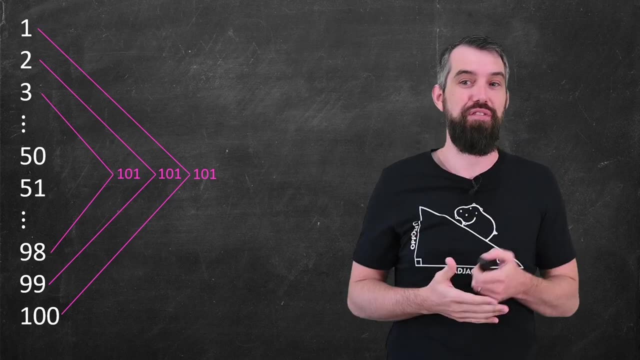 And what he did was notice that the first and last number- 1 and 100, adds up to 101. As does 2 and 99. As does 3 and 98. All the way down to the middle, where 50 and 51 also add up to 101. 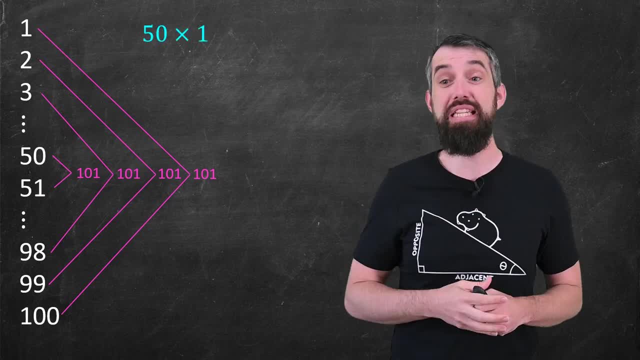 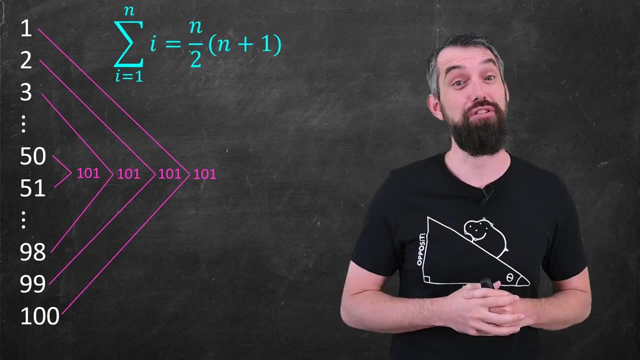 So as a result it's just 101,. well, 50 times, because only half of the numbers are needed to get each pairing. And then we can use summation notation to get this nice general result where the sum of the first n numbers 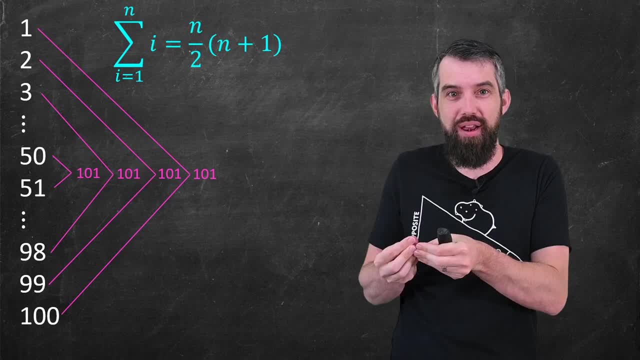 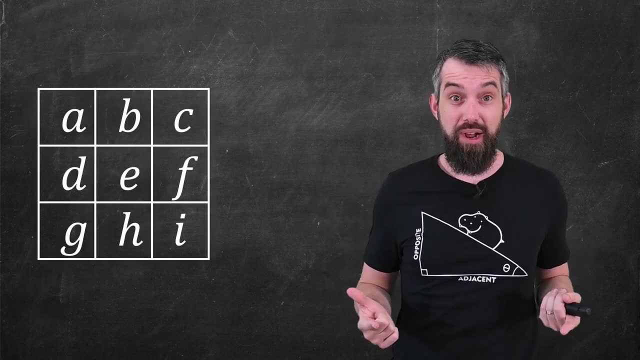 well, you take pairs of numbers and add them up to be n plus 1, and since it takes two things to make one pair, there's n divided by 2 copies of this n plus 1.. So let's prove our first lemma, that some of the rows, or the columns, or the diagonals, all add up to 15.. 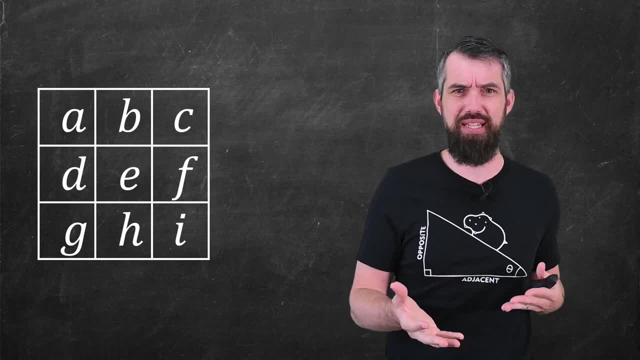 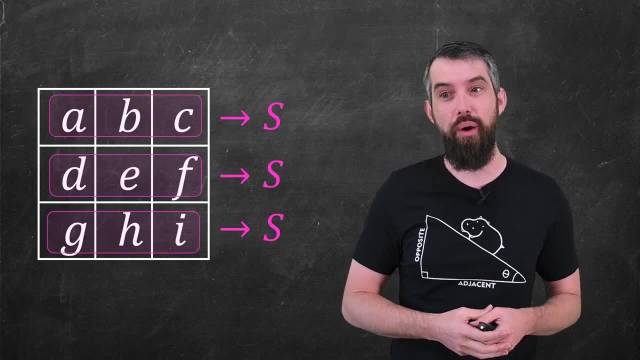 Well, if I leave it, generic ABC here is meant to say I haven't figured out which of those are 1,, which of those are 2, and so forth. But if I add up the first row, the second row and the third row, 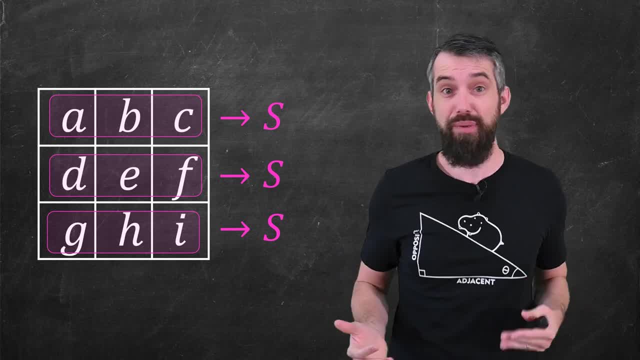 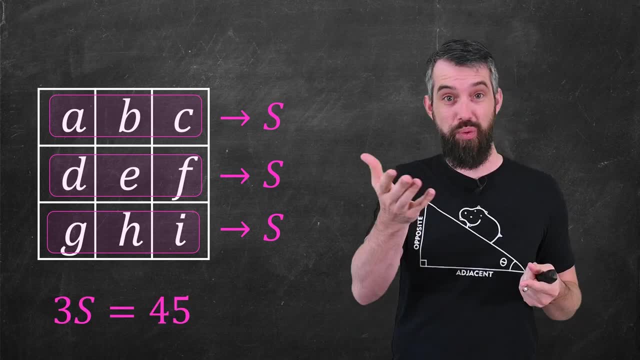 then I've got every single number once, As in, the sum of those three rows is every single number. So if I call the sum of a single row a generic number like s, that means that three copies of s better equal 45,. 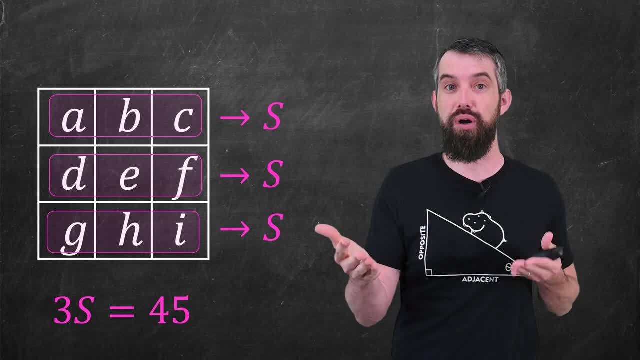 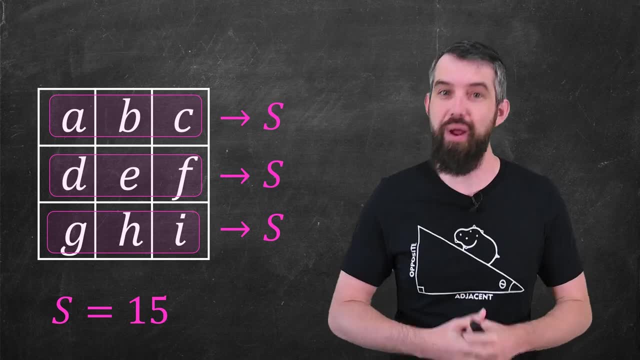 which is just the sum of the numbers between 1 and 9, as we computed earlier. If 3s is 45,, then s is 15.. The sum of all the rows is 15. And, by definition of the magic square, the sum of the columns and the main diagonals are also 15.. 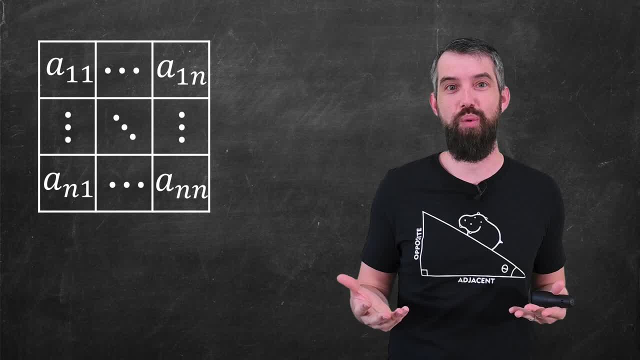 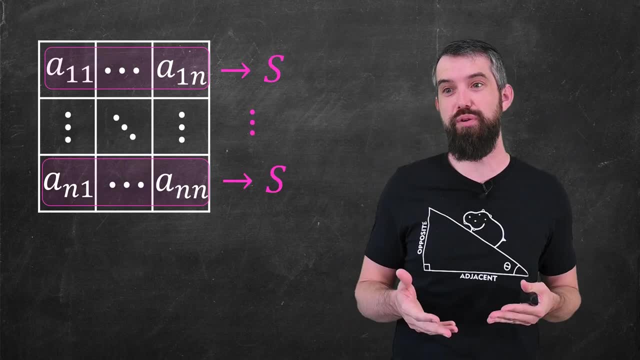 I can generalize this to an n by n magic square, just the same where? now I'm talking about the number between 1 and n squared. But again, if I look at the sum of all of the different rows, say each individual row is equal to s. 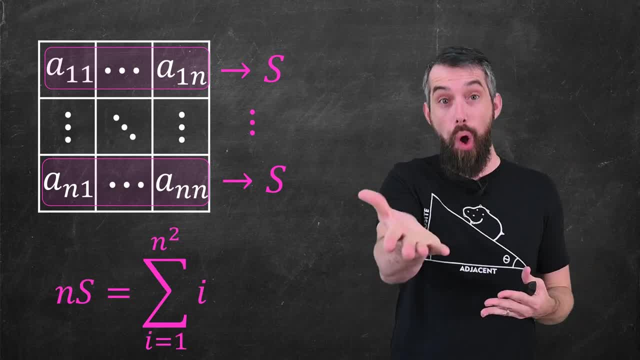 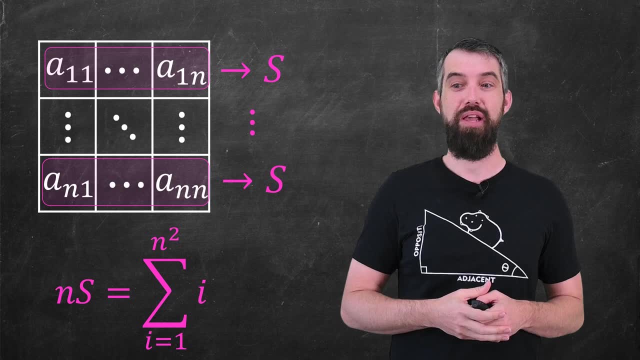 then what I have is n copies of s is all of the numbers between 1 and n squared added together, But by our formula I'm just plugging in n squared now. so this is the same thing as n squared, n squared plus 1 divided by 2.. 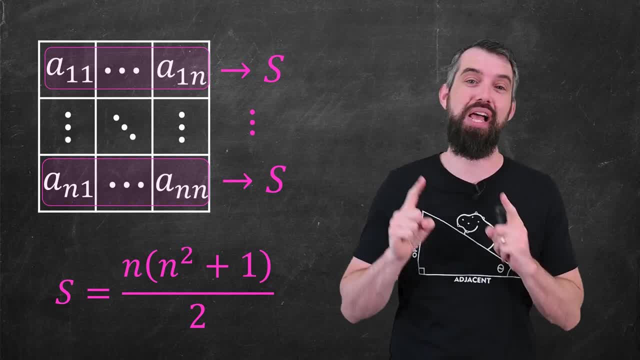 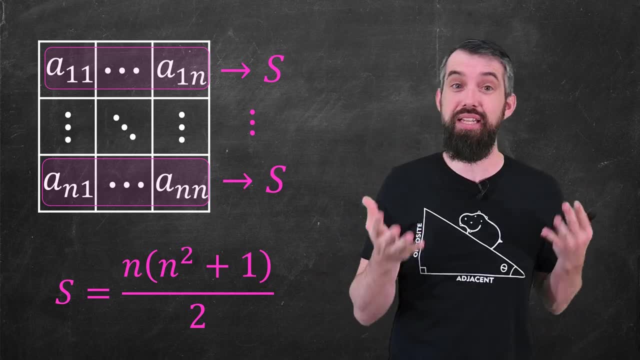 Cancel and end on both sides. And now I know that the sum is n? n times n squared plus 1 divided by 2.. For example, in the 4 by 4 case, 4 squared is 16 plus 1 is 17.. 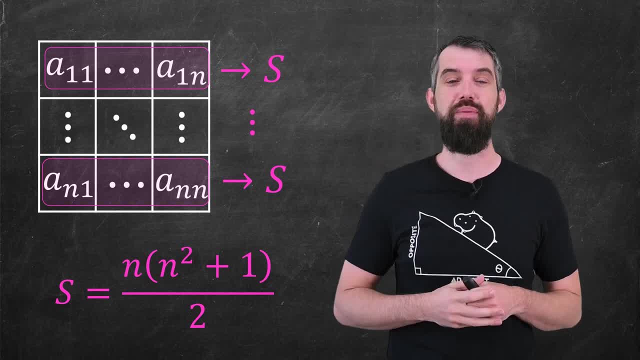 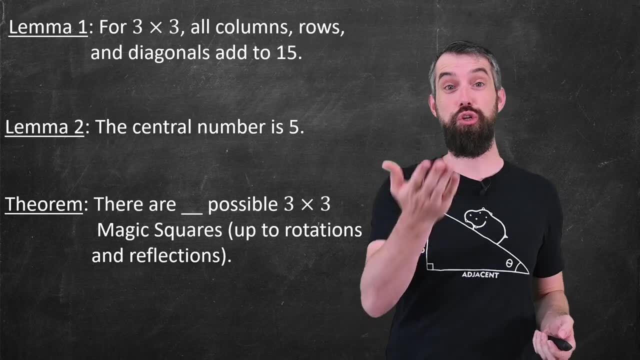 17 times 2 is 34.. So, as we saw in our earlier image, the sum of every row and column in the main diagonals in a 4 by 4 case is 34.. Alright, so we have managed to prove our first lemma. 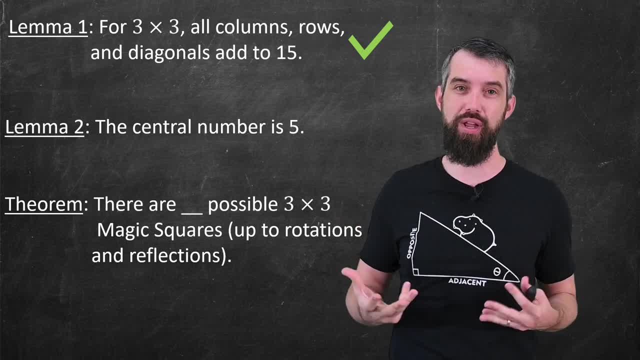 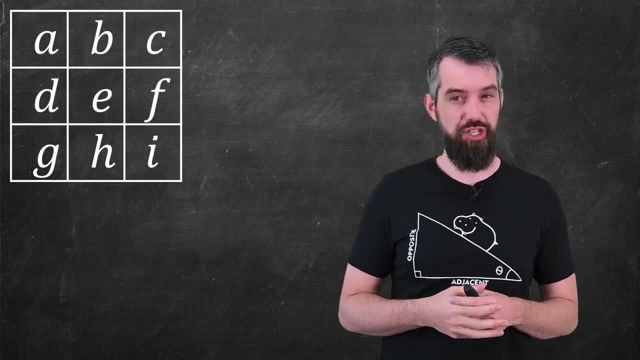 and we even talked about how this first lemma generalizes to the 4 by 4 case. Next lemma is about the center number being 5.. I'm going to do a similar trick. I'm going to start with a generic number, A generic magic square here. 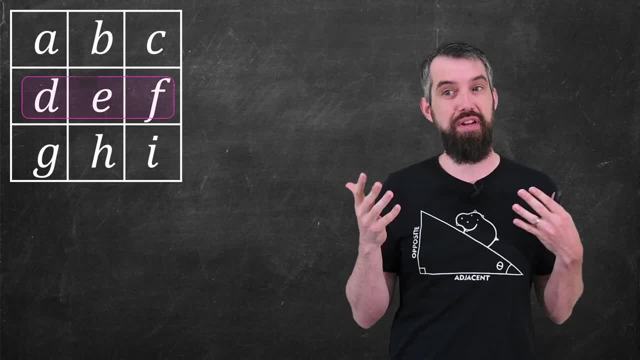 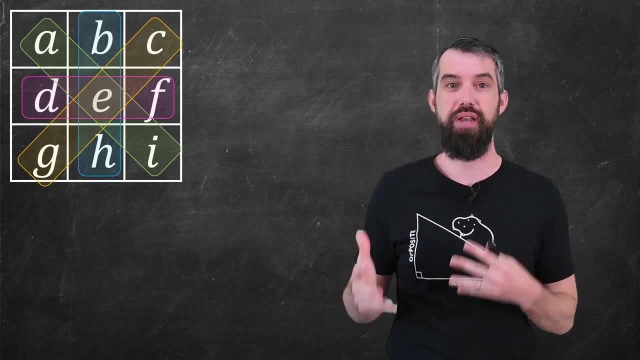 And then I'm going to think about every row, every column or every diagonal that intersects with that central number. That includes the e, which is my placeholder for this center number. Okay, so if I add all of those 4 things up, 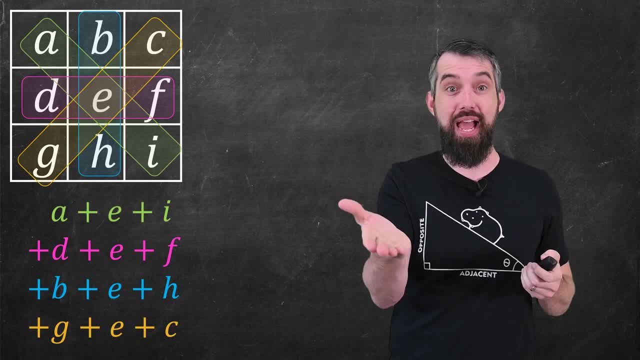 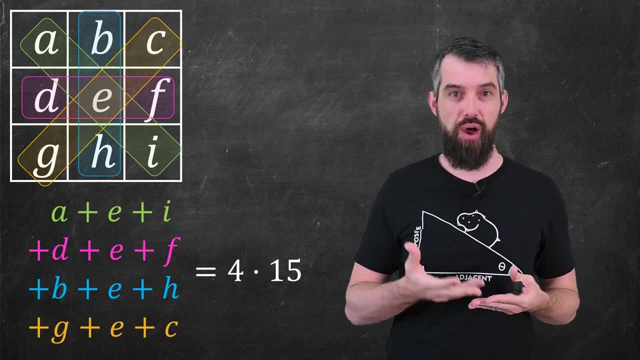 I'm adding 4 different rows, columns or diagonals, So this better equal to 4 times 15.. We've already decided that 15 was the number that has to be for all these rows, columns and diagonals. And then, if I look at the letters, 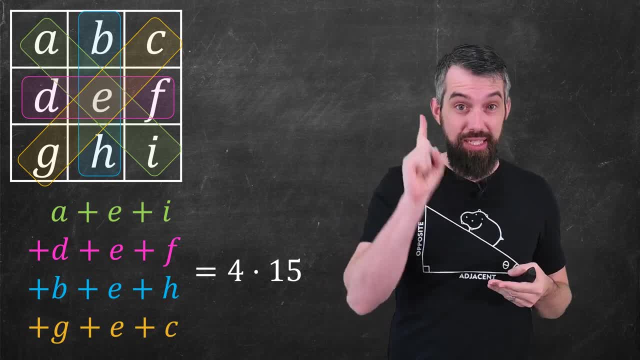 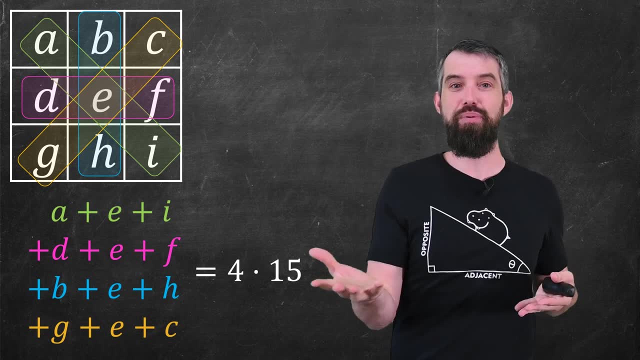 I notice that every 1 between the 1st and the 9th is used exactly once, with the exception of e, that's used 4 times. Or another way to say this is: every number is used exactly once, and then the thing in the middle has 3 additional usages. when I write it this way, 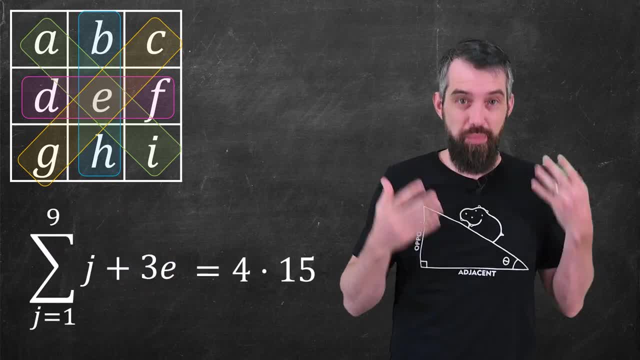 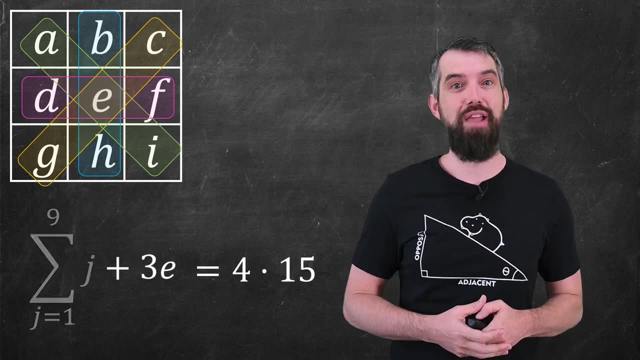 So that is to say that the sum of the first numbers plus 3 times e is equal to, well, 4 copies of 15 or 60. So I can compute that out: That was just 45. This leaves me with 3e being 15,. 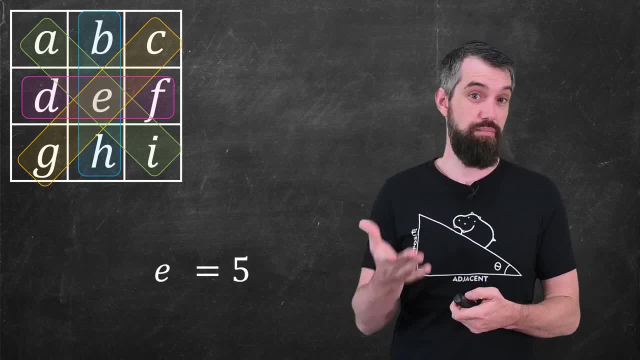 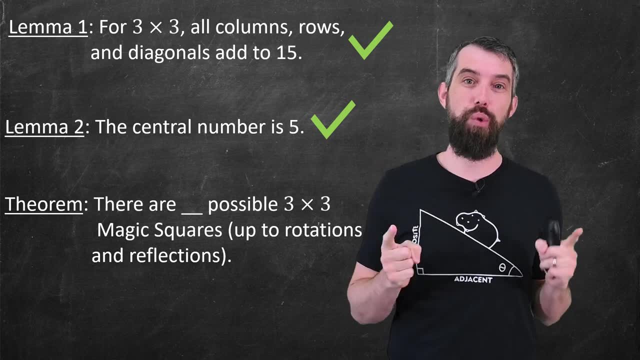 and now I've deduced, e has to be 5.. And so we showed our second lemma: The central number is just 5.. Okay, now to my theorem. I want to use these lemmas to figure out the total number of 3 by 3 magic squares. 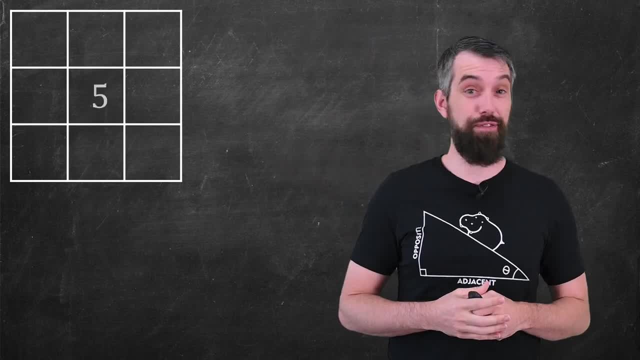 Let's start with a generic grid. We know the center point, That's a 5. We can fill that in already. Let me conjecture that I was to put a 1 in a corner. Could be any of the 4 corners. 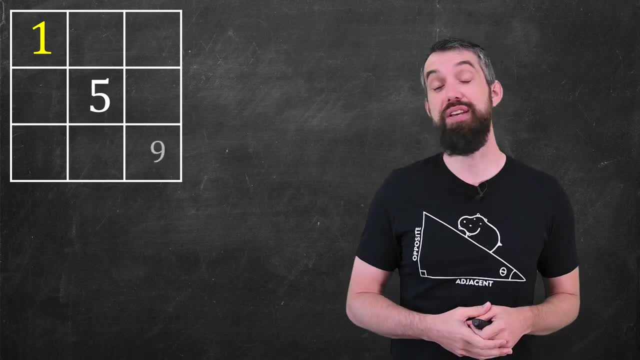 I'll do this one Going along that diagonal. that means I have to have a 9 in the final spot, 2.. I need to be able to add up to 15.. Now let's think about the top row. It's got a 1 in it. 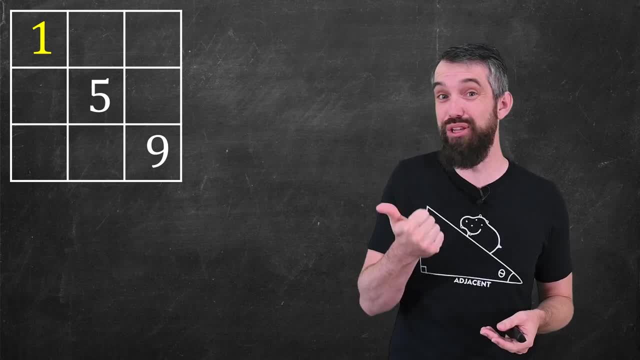 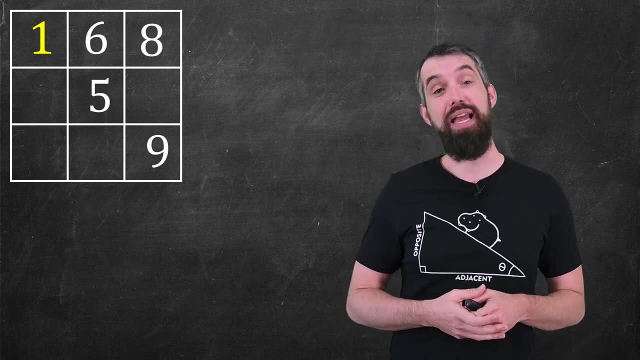 So the other two numbers better add up to 14.. Can include a 9. Can include 7 plus 7. That would be a repetition. So there's only two possibilities: It could be 6 and 8. Or it could be 8 and 6.. 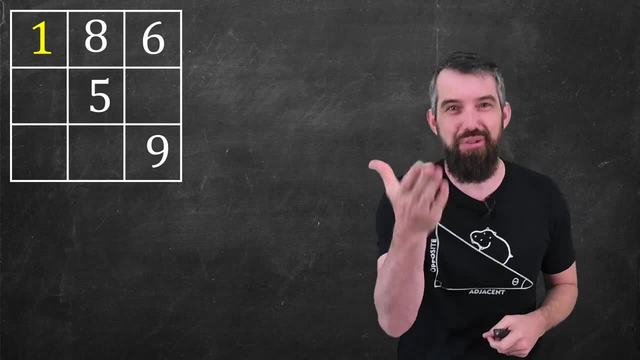 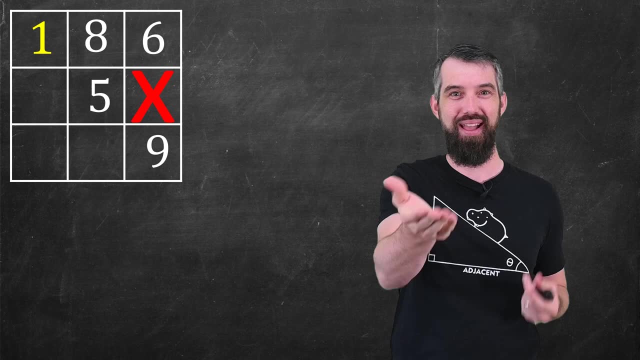 Those are the two possibilities for that top row, But neither of these is valid, Because if I now look at the far right row, well, 6 and 9 is already 15.. I'd have to put a 0 in, And if the 6 and the 8 swap, 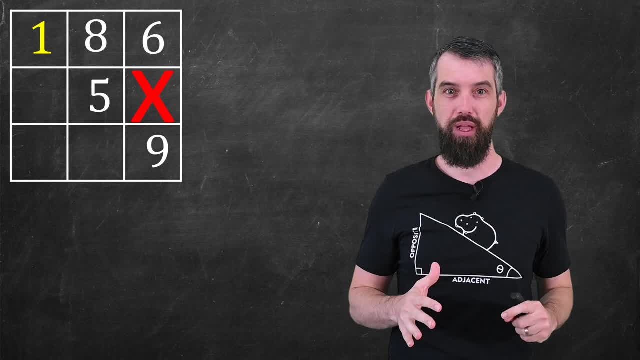 it would be even worse. I'd have to put a negative number in. Neither is possible. And if I put the 1 in any of the other corners, the same problem happens. You cannot put a 1 in the corner, Okay. 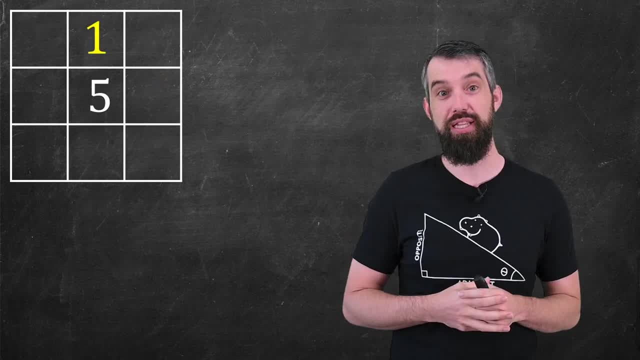 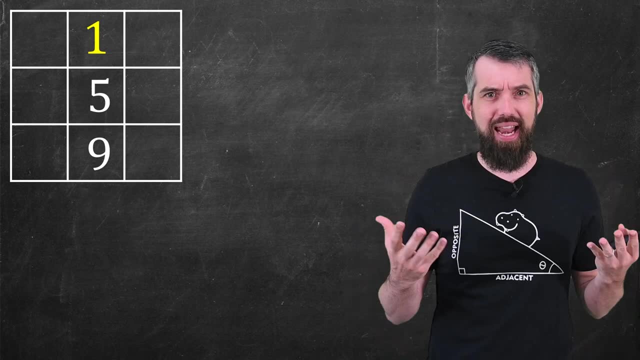 So let's put the 1 in one of those middle outside locations Like this one. Same story: 1, 5, 9 has to add up. And let's again look at that top row. Again. it has to be either 6 and 8 or 8 and 6.. 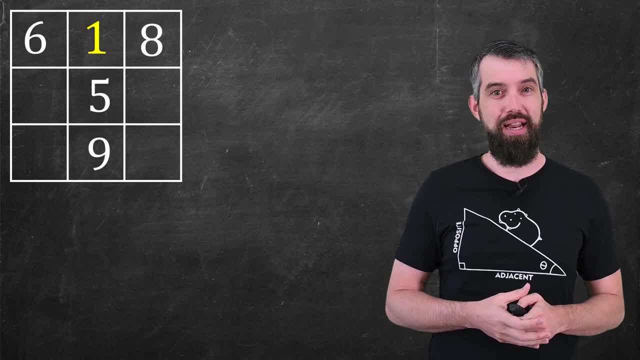 So how about I do it this way? 1 I'm going to write down is 6 and 8. And then I'm actually going to copy it over and do 8 and 6.. I'm going to do both of these at the same time. 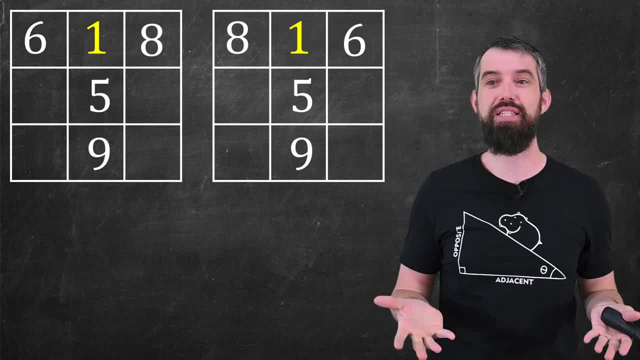 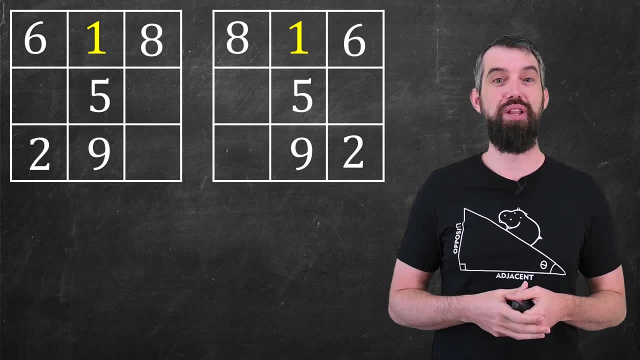 So I had a choice here. But after this choice everything is fixed Right. Going down that 8, 5 diagonal means there's a 2 in the opposite diagonal. Then I've got the 2 and the 9. And that's going to mean a 4 along the bottom. 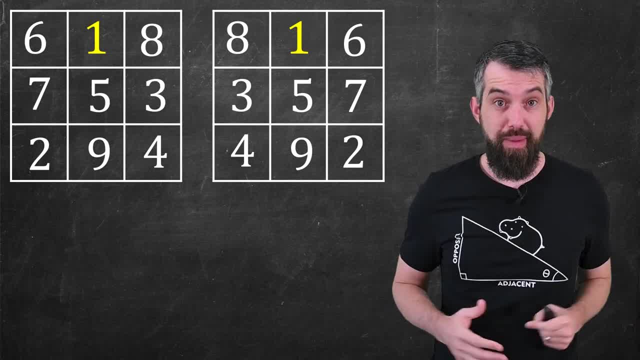 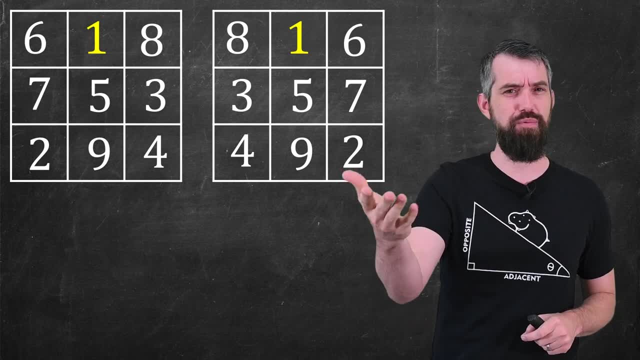 And I can fill in the 7 and the 3 as well. Both of these are magic squares, So they're two bonafide answers. But you noticed I had that little bit in there about up to reflection and rotation. Well, this is what I mean. 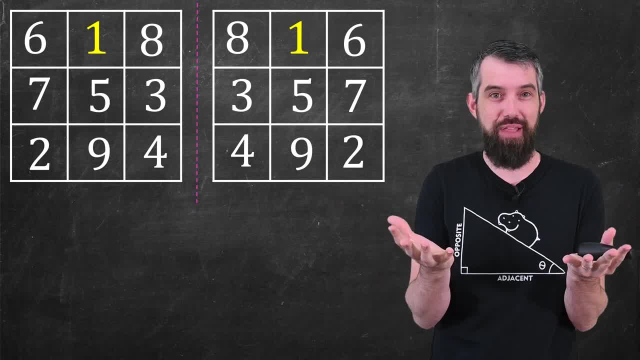 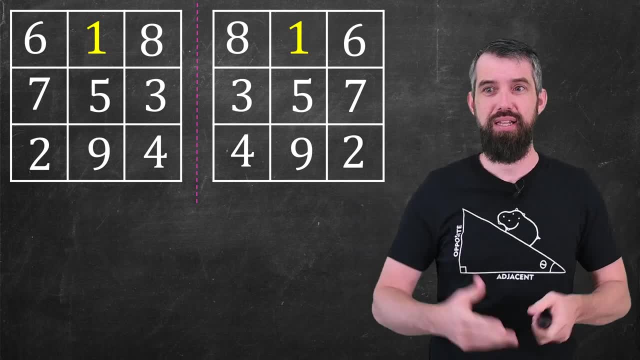 These two magic squares are just reflections of each other. So if I get rid of thinking about reflections then they're just the same magic square. Sort of up to reflections, It's the same story. if I consider one of them. I could just rotate the numbers so that the 1 is in a different middle location. 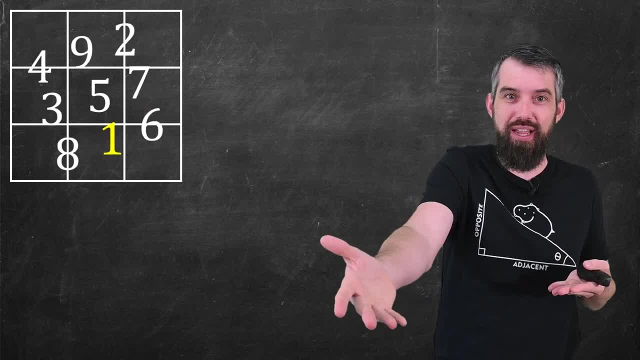 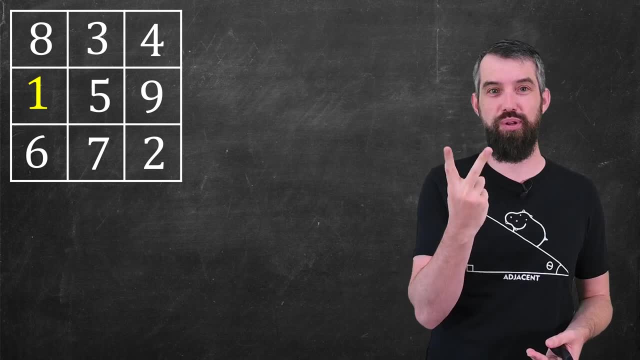 And so the idea is that, up to rotation, all of these things are exactly the same And, as a result, because there's four possible middle locations for the 1, and then two possible 6,- 8 pairs for each of those, 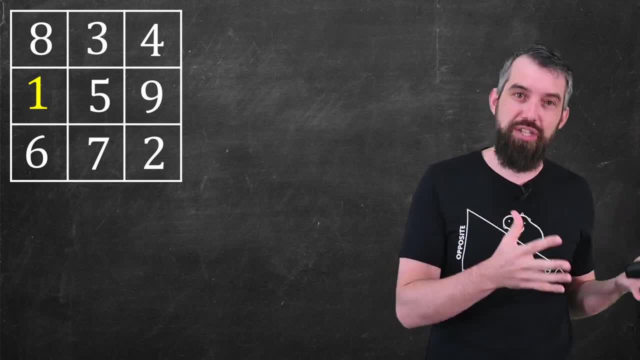 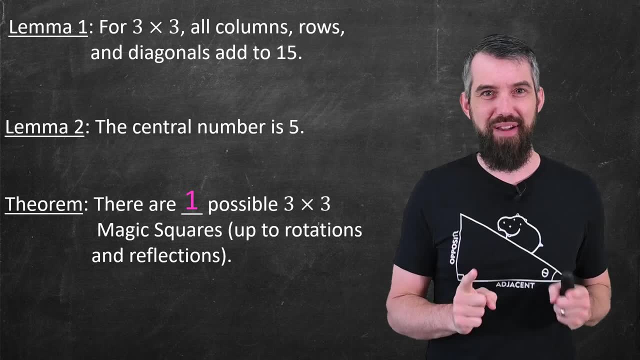 there's sort of 8 magic squares, But if you ignore rotations and reflections, we get to our final result. There is one possible 3 by 3 magic square, And what I find crazy about this is that, while this was simple for 3 by 3,, 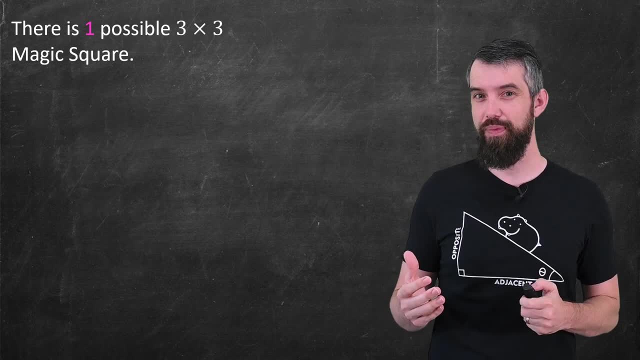 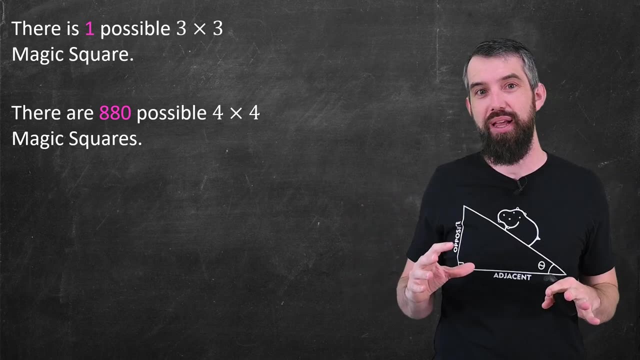 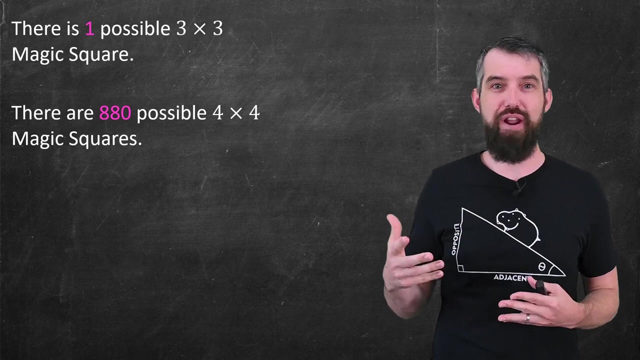 look how quickly this gets complicated. For 4 by 4, there are 880 possible magic squares. It's way less prescribed. We have seen one lemma already in terms of the sum of the rows being 34. And you can play around and try to find other things. that must be true about 4 by 4s. 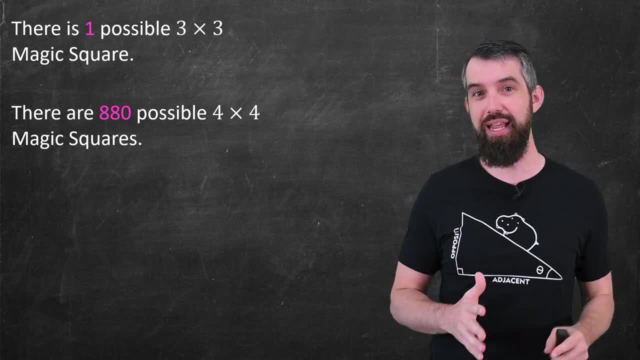 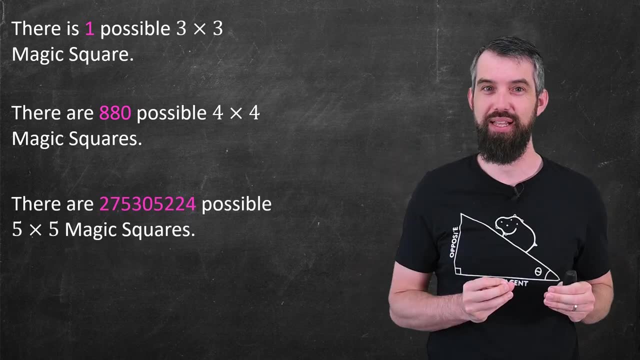 but there's way more options. Turns out 880.. And it grows fast. Like for a 5 by 5, there's 275 million possibilities. And- here's my favorite part- For 6 by 6, we do not know. 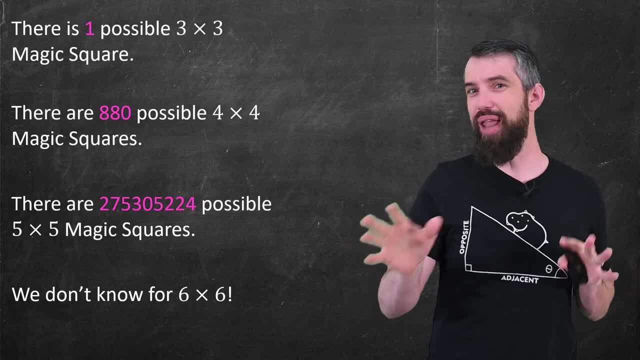 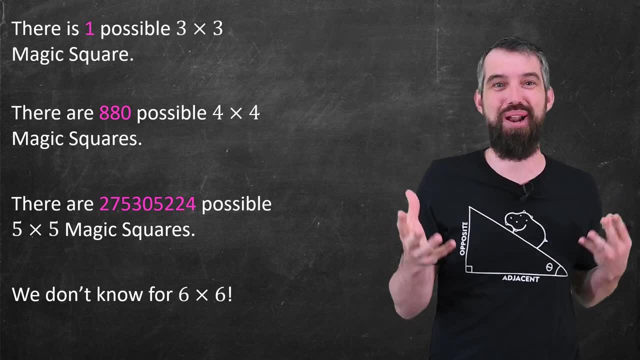 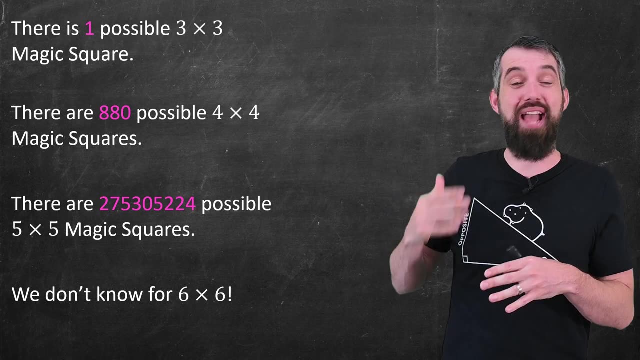 The number is so gargantuan- like statistical estimates sort of estimated around 10 to the 19,- that we don't actually have a way to mechanistically compute it out on our computers so far. It's just too big, And so magic squares start extremely simple and get really complicated. 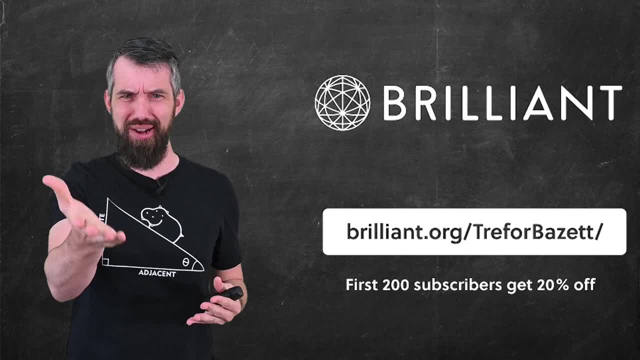 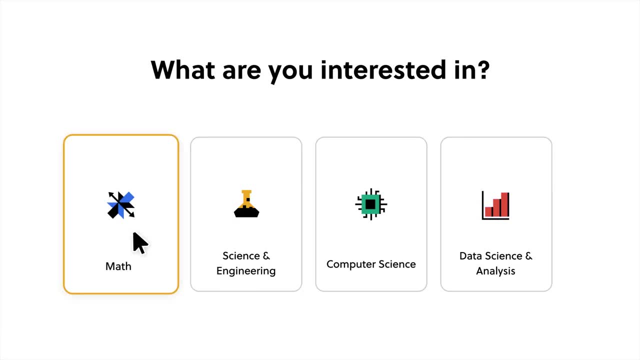 Now, if you enjoyed this video and want to learn today's math puzzles and want to do more, want to get better at math, then I strongly recommend today's sponsor, Brilliantorg. Brilliant is an online learning platform with thousands of lessons.